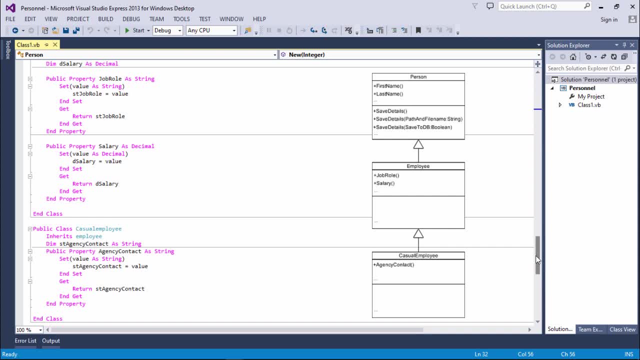 The arrows indicate inheritance. So the diagram clearly shows that the casual employee has an agency contact, a job, role, salary, first name, last name and three overloads of the saveDetails method. You can imagine that there are lots of other properties specific to an employee which we could write code for in the employee class, such as: 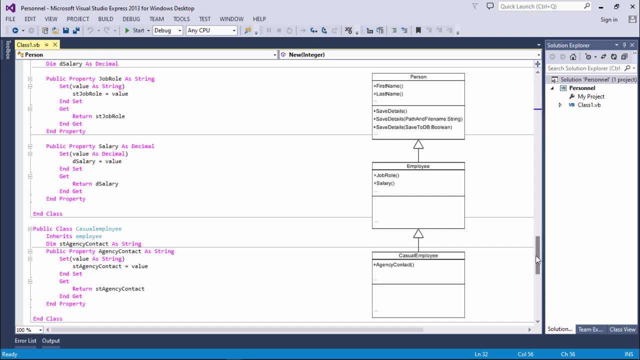 The name of their supervisor, The date they started working at the cattery, How many years of experience they have working with cats, Their cat care qualification And whatever other properties a cattery employee might have. If all of these extra properties were coded into the employee class, the casual employee would automatically inherit them. 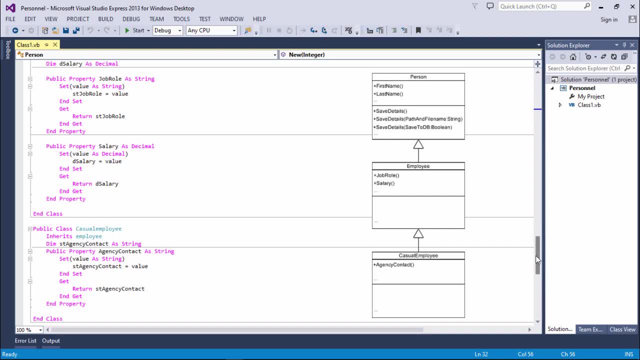 That's the power of inheritance. To put it another way, any public properties that make up the public interface of the employee class automatically become part of the interface of the casual employee class. Make sure you're comfortable with this idea before you continue. 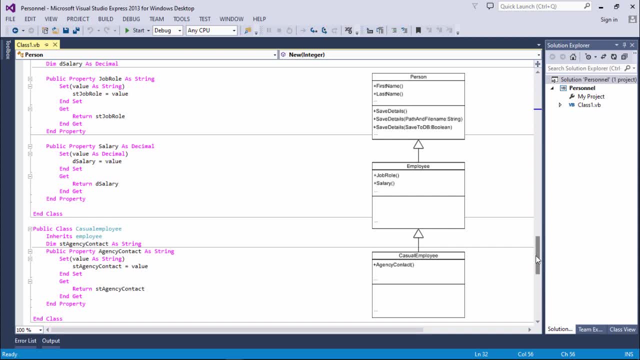 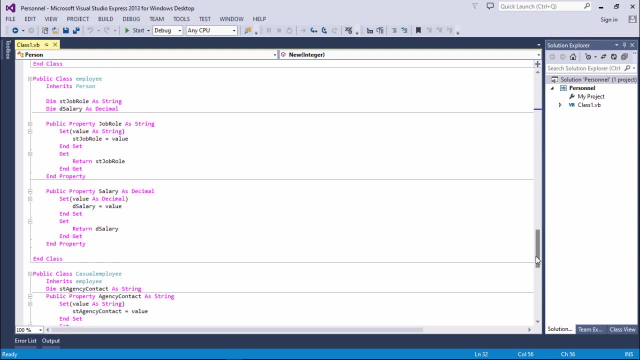 If not, review the other videos in the series. Now, arguably, the code you can see here is flawed Because I've put a salary property in the employee class. Why? Well, it comes down to how you define the word salary. 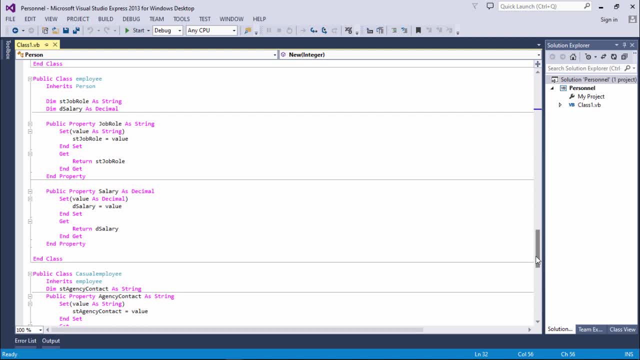 A full-time permanent employee would probably have a salary- A fixed amount, paid each month into their bank account according to their annual salary. For example, if their annual salary was £24,000, they would get £2,000 per calendar month. Minus deductions like tax. A casual employee, on the other hand, is more likely to be paid for the hours they work each week or month multiplied by an hourly rate. For example, if they work 25 hours in a month at £10 an hour. 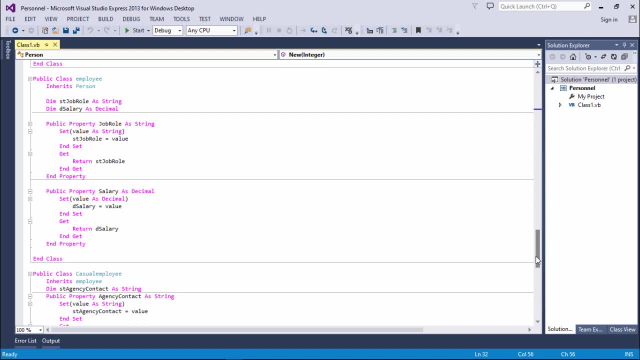 they would get £250.. But our casual employee has inherited the salary property, Which is inappropriate. There's an important point to be made about inheritance here. A subclass can't selectively inherit just some of the methods and properties of its superclass. It will inherit them all. 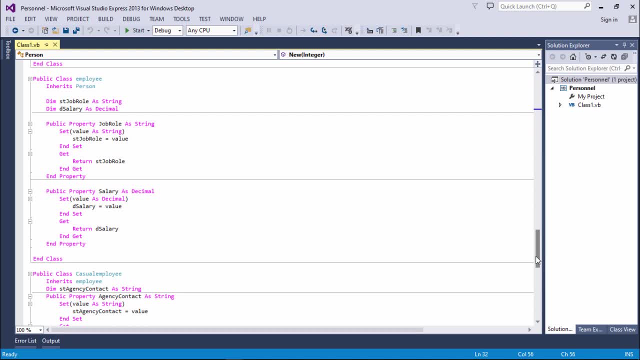 In an attempt to put this right, I'm going to rename the salary property in the employee class to something more generic, Let's say Rate of Pay. So this change is now automatically inherited by the casual employee class. Here it is on our class diagram. 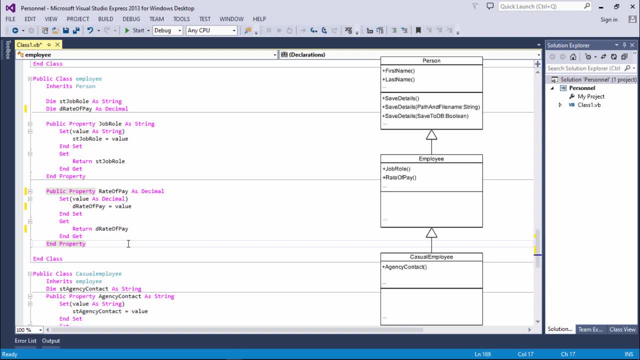 When I assign a value to the Rate of Pay property for a permanent employee, I need to be aware that it will be their annual salary. When I assign a value to Rate of Pay for a casual employee, I need to be aware that it will be their hourly rate. 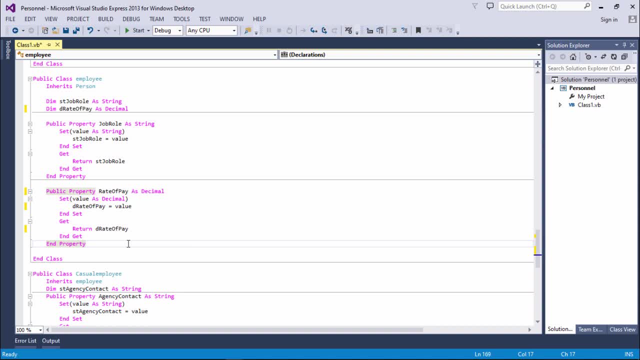 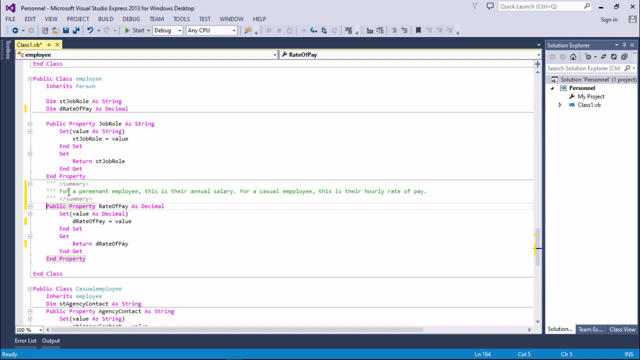 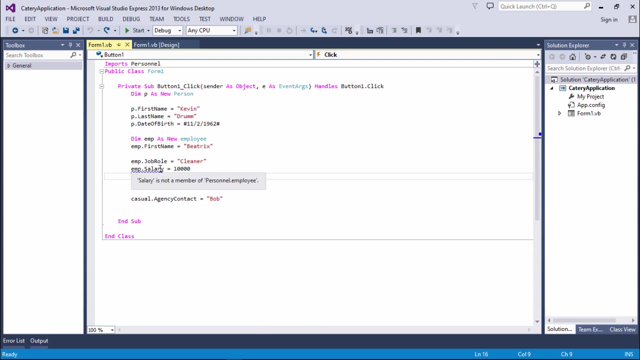 Here's a neat little feature in VBnet that I can use to make this clear in the front end. Let's rebuild the class library and see how it looks in the front end. I have a compiler error now because there is no longer a salary property. 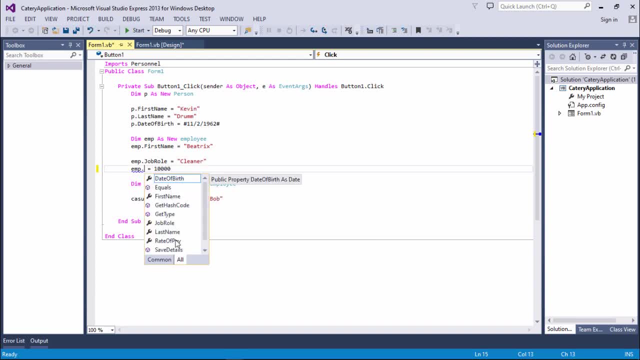 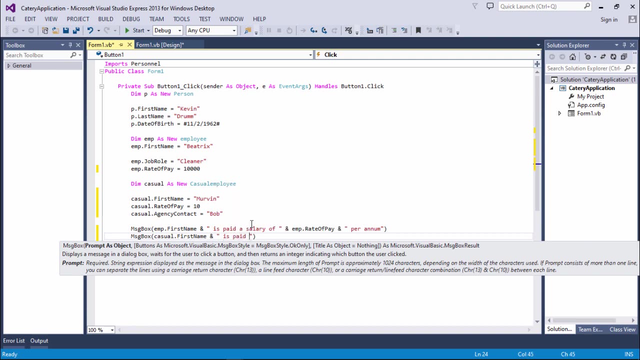 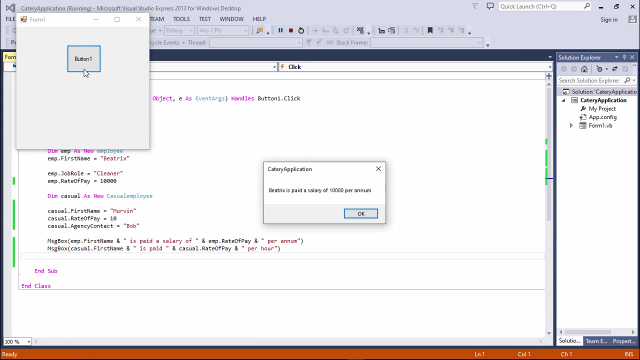 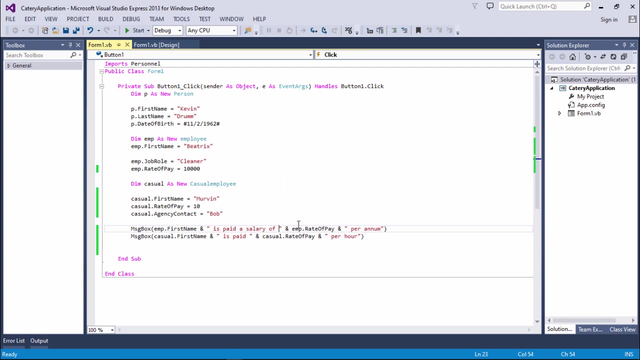 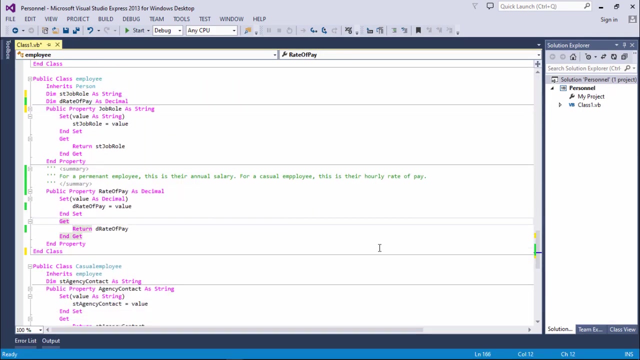 It's called Rate of Pay, And there it is, And you can see the description I've put on there as well, Making it clear how to use this. Thanks for watching. I'll see you in the next video And I think I'll give Beatrix a pay rise. 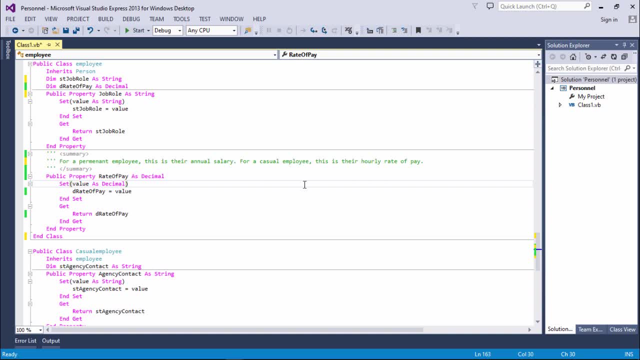 Now, arguably a better approach would be to have an employee class with all of the properties that are common to any type of employee – start date, supervisor, qualification – but not salary. Then to have a separate permanent employee class with a salary and a separate casual. 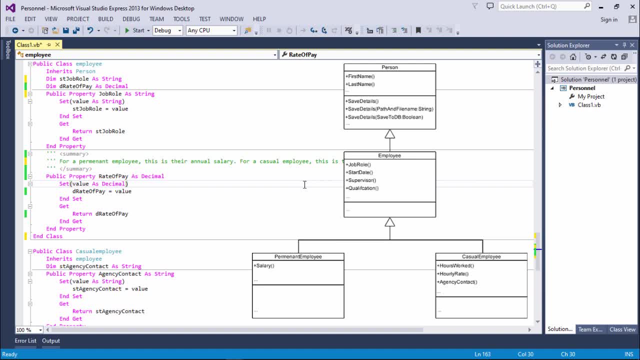 employee class with an hourly rate and the number of hours worked. Both types of employees would then inherit from the more generic employee class. Nevertheless, let's proceed with the original approach. My casual employee now needs an hours worked property so it can be used along with their 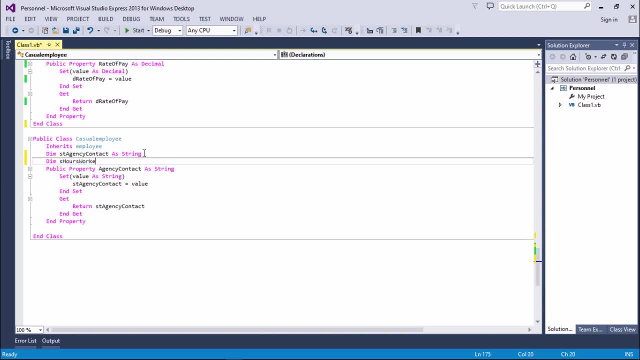 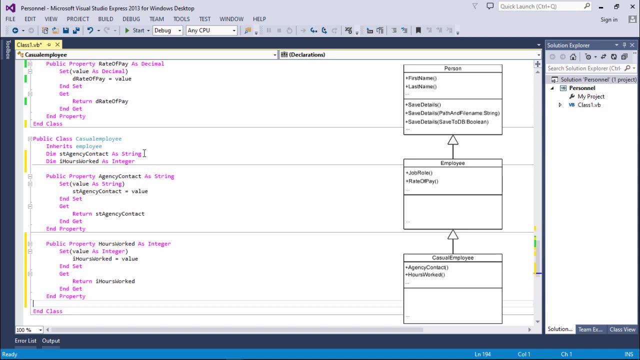 rate of pay to calculate their wages. I could use a single, but I'm going to use an integer, because in this cattery you can only work a whole number of hours. Here's the change in my UML class diagram. Now let's talk about polymorphism, perhaps the least well understood feature of object. 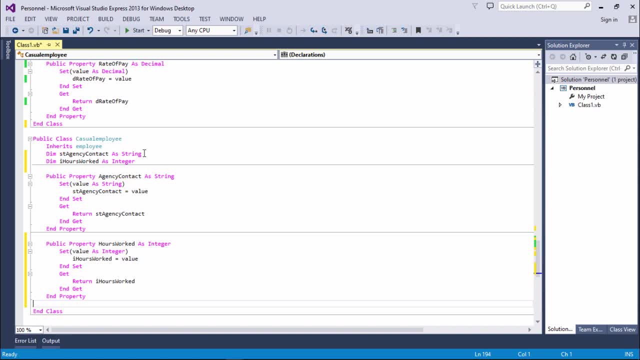 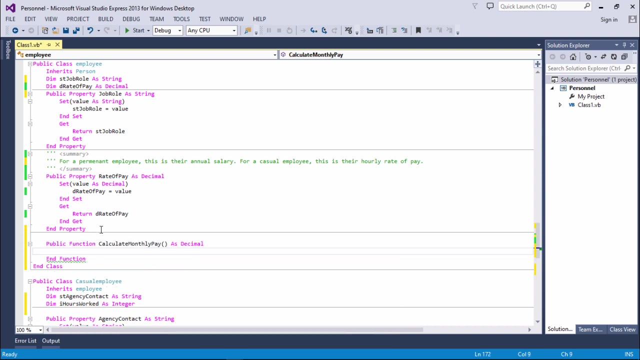 oriented programming. I'm going to code up a calculate monthly pay method in the employee class. This will take the rate of pay, which for a permanent employee is their annual salary, and divide it by 12 to get a monthly amount. Decimal is the best data type when you're working with money. 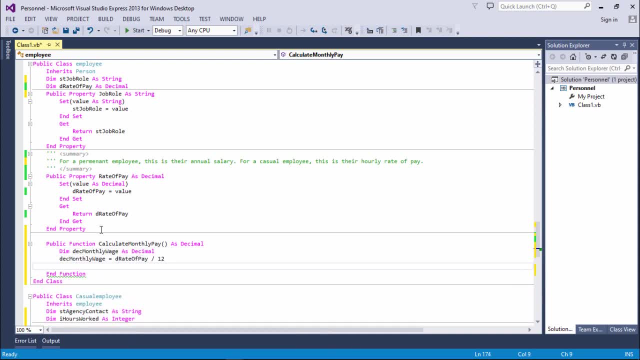 I could of course include code to make deductions for tax and pension contributions. In fact, the result of the calculation would probably get saved to a payroll database and then trigger a bank payment. But that's beside the point. For the purposes of this demonstration, my method will just return the result of a simple 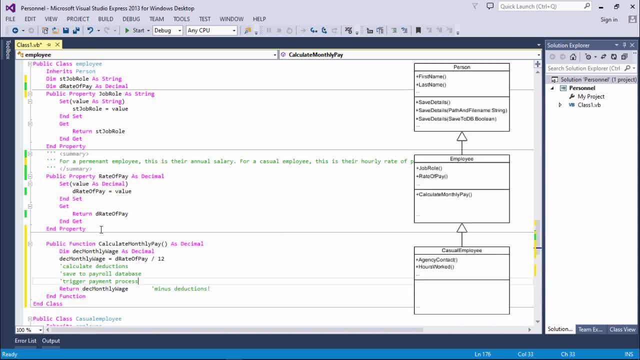 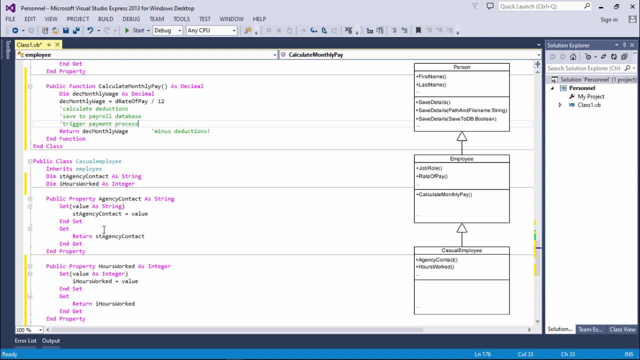 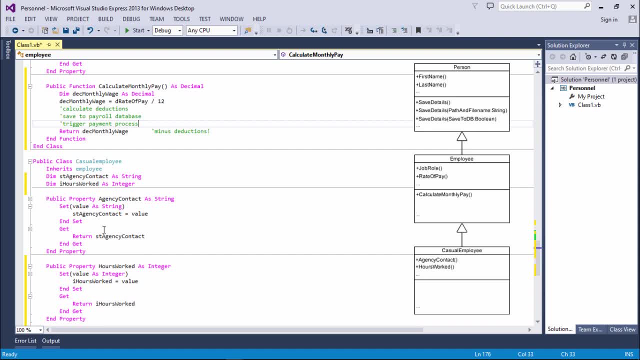 But what the method does is totally inappropriate for a casual employee. I want the casual employee class to have a calculate monthly pay method too, but I want it to do something completely different, namely multiply the rate of pay by the number of hours worked. 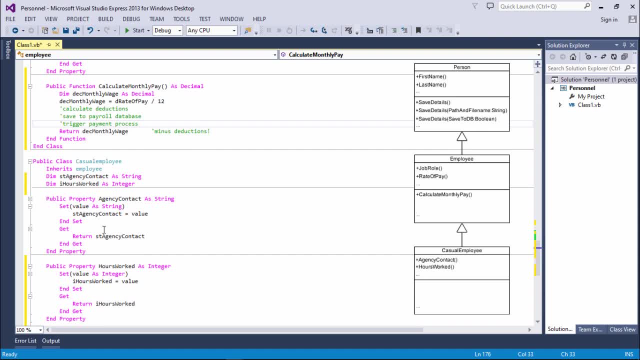 I want the casual employee class to replace or override the calculate monthly pay method that it inherited. I want the casual employee class to replace or override the calculate monthly pay method that it inherited. In this case, it has to Mỹ exceed Restaurant expected pay. 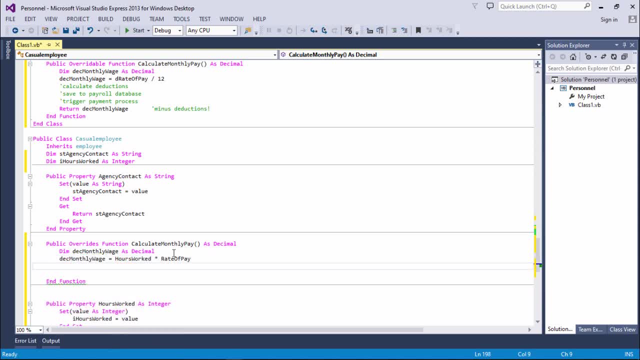 The most crucial part of the calculation, however, was the quantity. To do this, I need to indicate that the superclass method is overridable. Now I can override it in the subclass using overrides. Notice that the most crucial part of the calculation is different for the employee, however. 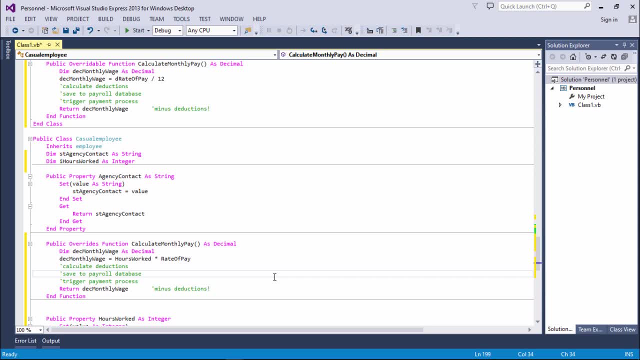 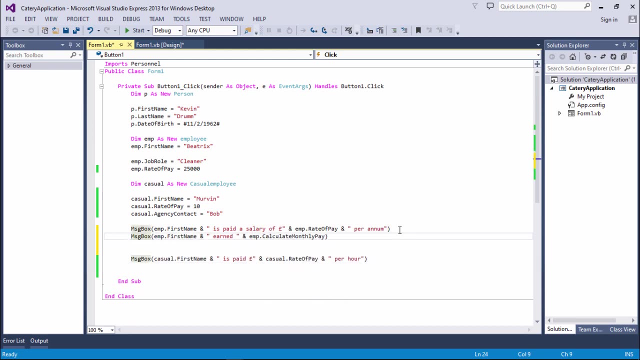 I'll do that, inya. I'll take a пользов��kas bela. capture inya under ket and the casual employee. let's see what happens in the front end. there's the method call for the permanent employee and there it is for the casual employee. 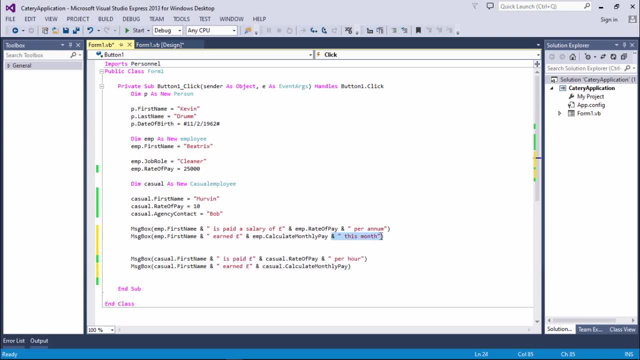 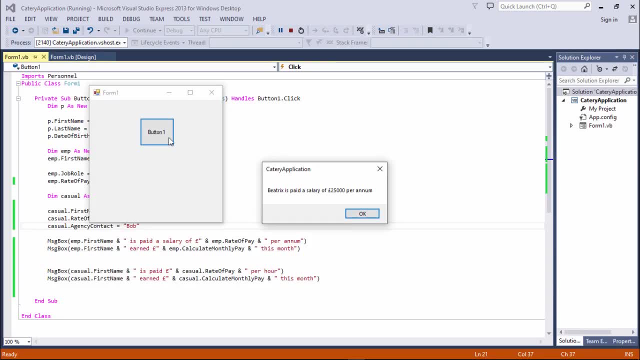 a little bit of tidying up of the output. Beatrix is paid a salary of twenty five thousand pounds per annum. Beatrix owned well about two thousand pounds this month. I could do with wrapping up that method. call in a format function to get rid of some of those decimal places. Mervyn is paid ten pounds. 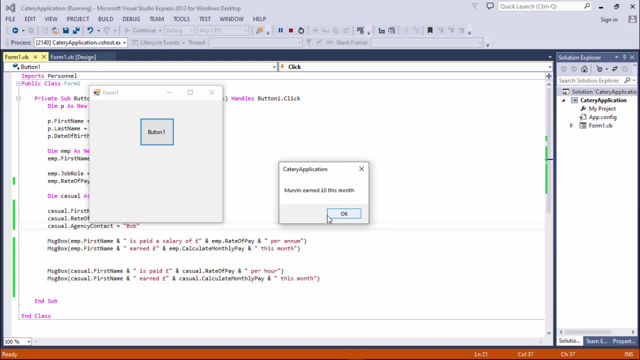 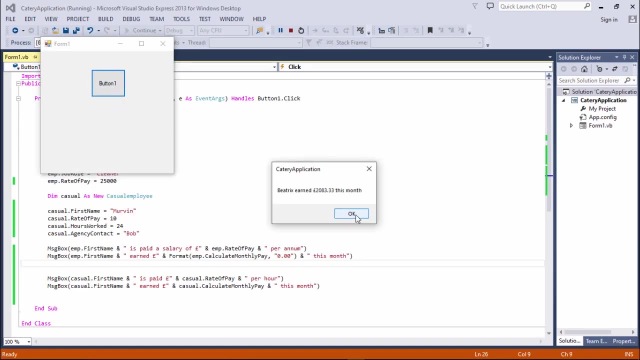 per annum, and then Beatrix is paid a salary of twenty five thousand pounds per annum and then hour and Mervyn earned zero pounds this month. I think the problem here is that Mervyn hasn't worked any hours. let's fix that. that's better and Mervyn's made some. 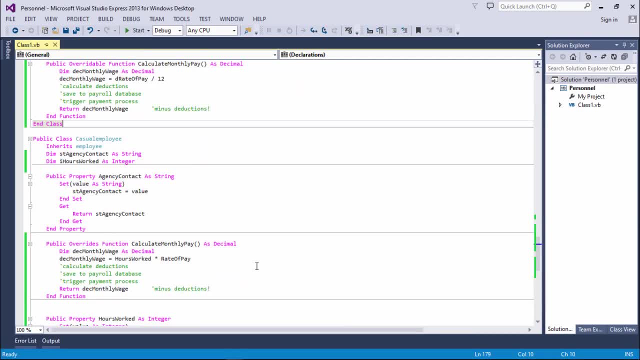 money as well. so what we have here are two different forms of an employee object behaving differently. when a method with the same name is called, two different types of employee have the same interface, but they implement it in different ways. we call this polymorphism. literally, poly means many and morph. 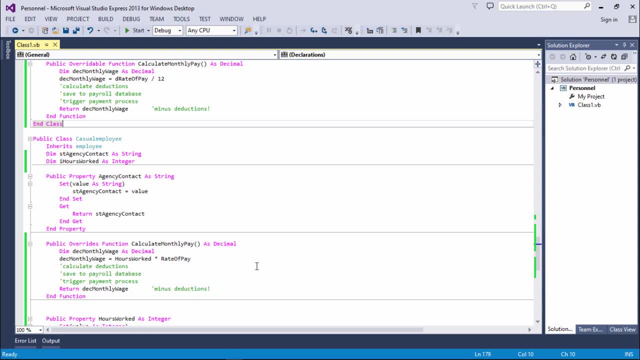 means form. to put it more simply, an example of polymorphism is when a subclass overrides a method that it inherited from a superclass. here's an updated class diagram. the simple fact that the same method appears in the superclass and the subclass indicates that the subclass has overridden it. if overriding a method is an example of polymorphism, 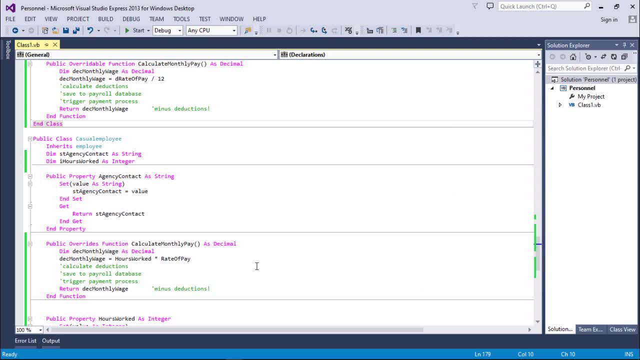 what's another example of polymorphism. another example of polymorphism is when a subclass overloads an inherited method. in the previous video, you saw how to overload a method within the same class by creating multiple variations, each with a unique method signature. well, it's also possible for a subclass to overload a method that it inherited a subclass. 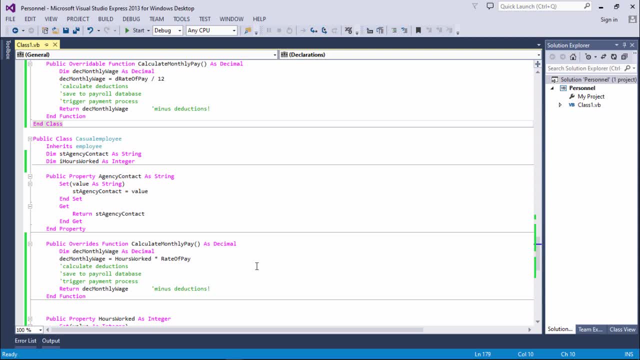 can have its own extra variations of an inherited method. for example, let's put a method in the employee class that can be called when we want to pay a hard-working employee a bonus. for example, let's put a method in the employee class that can be called when we want to pay a hard-working employee a bonus. notice how the employee is calling its own calculate monthly pay method and then getting 10% of this. if a permanent employee gets a bonus, it will always be 10% of their monthly pay. this method is now automatically inherited by the casual employee and the casual employees bonus. method will call its own calculate monthly pay method. so the casual employee's bonus will be 10% of their rate of pay multiplied by the number of hours they work. let's quickly check. Beatrix earned a bonus of 208 pounds. again, we could do with formatting that. 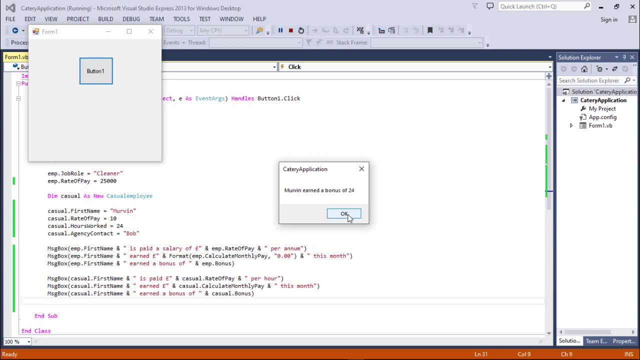 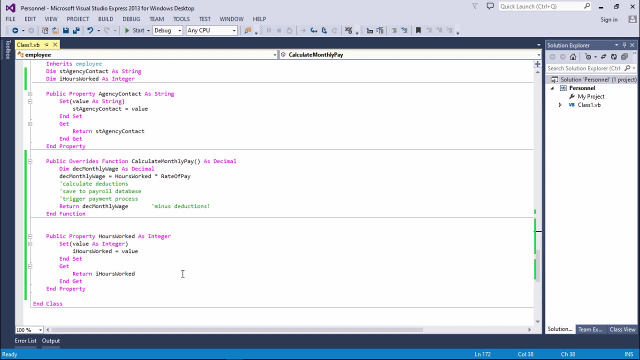 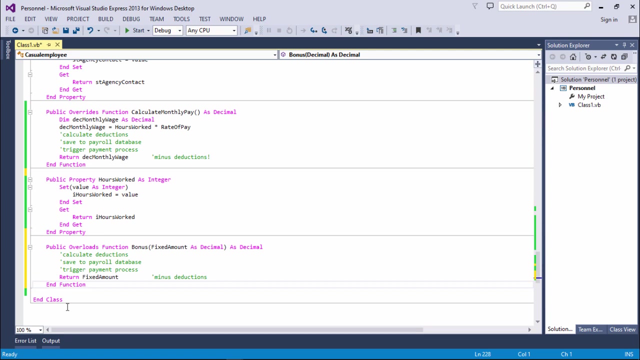 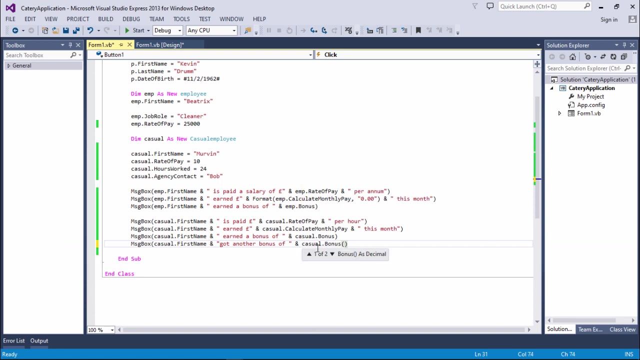 Mervyn, on the other hand, earned a bonus of 24 pounds. that's working fine. now let's suppose that a casual employee could also be paid a fixed amount of, say, five pounds, rather than a proportion of their monthly wage. you let's take a look at the front end and notice that the casual employee has got 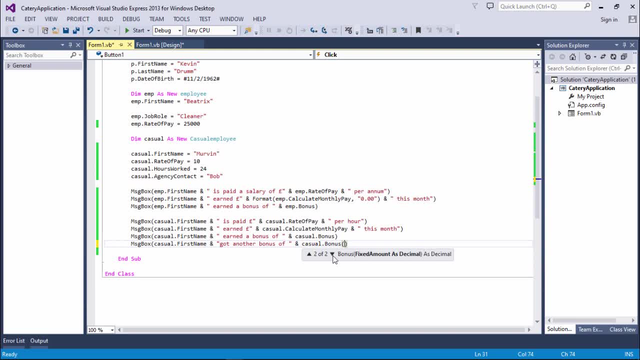 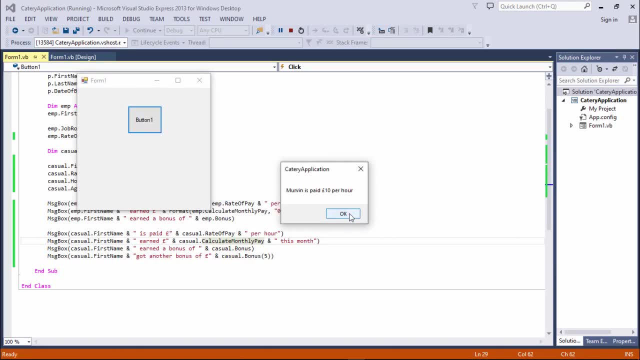 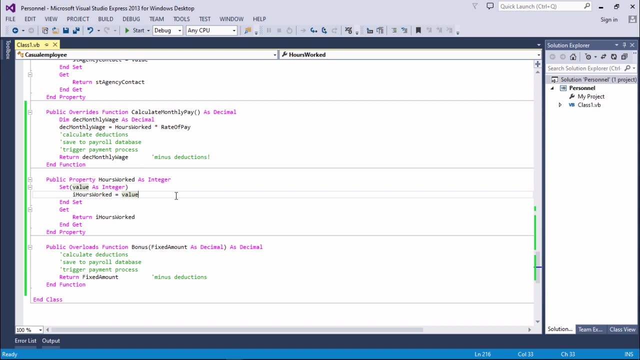 two versions of the bonus method: one with a parameter and one without lucky Mervyn again you can see, now that the casual employee has got, two versions of the bonus method: one with a parameter and one without lucky Mervyn, again you can see multiple forms of an object, namely an employee behaving differently. 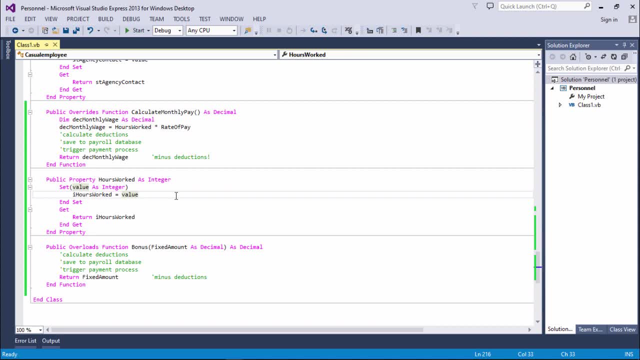 polymorphism is exemplified by a subclass overriding or overloading an inherited method. here's an updated diagram. notice that bonus appears in the superclass and the subclass, but the fact that the method signatures are different means that an inherited method is being overloaded rather than overwritten. Mervyn again, you can see that the casual employee has got two versions of the bonus method, one with a parameter and one without lucky Mervyn again. you can see that the